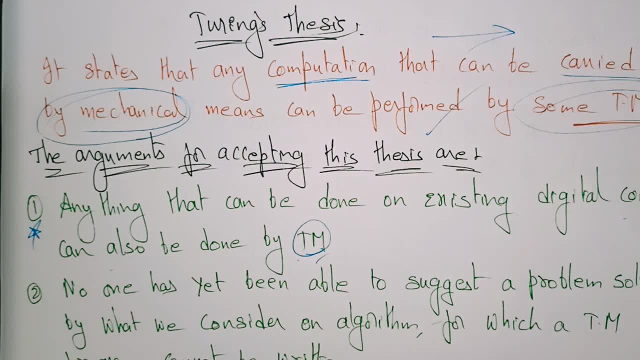 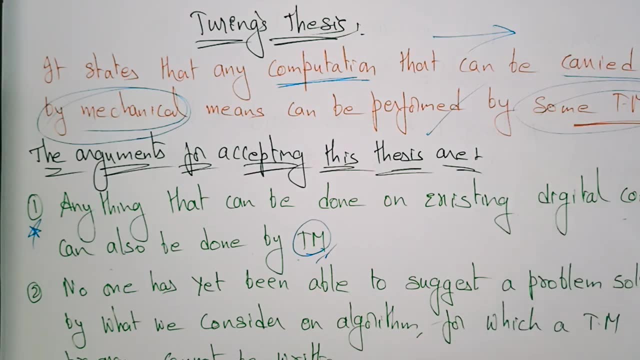 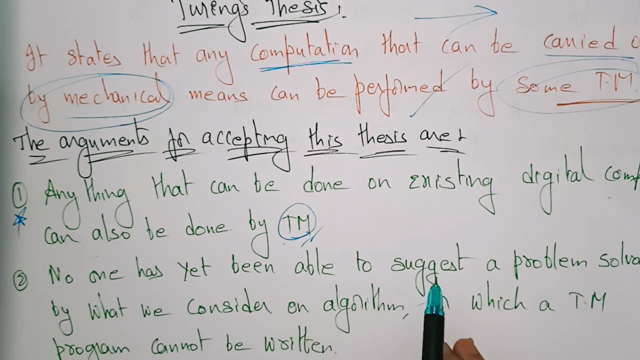 that can be done on existing digital computer. it can also be done in turing machine. so this is how efficient, compared to the digital computer, the turing machine is also the efficient. and here no one, no one has been able to suggest a problem solvable by what we consider on algorithms, for which 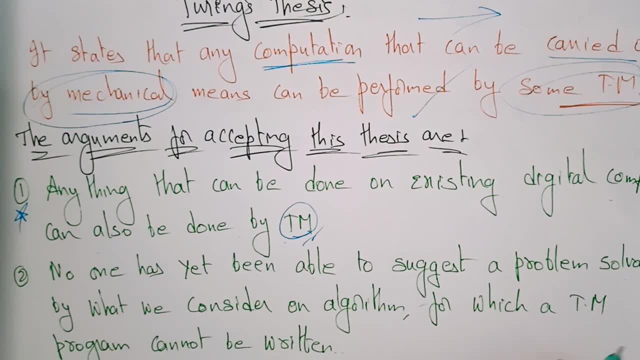 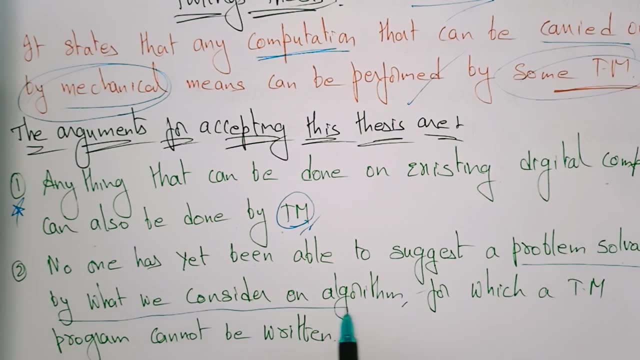 a turing machine program cannot be written. okay, so no one has been able to suggest. they are not able to suggest also a problem that is solved by considering an algorithm. by considering any algorithm you solve some problem, but no one has it been suggested for which turing machine program cannot be written. 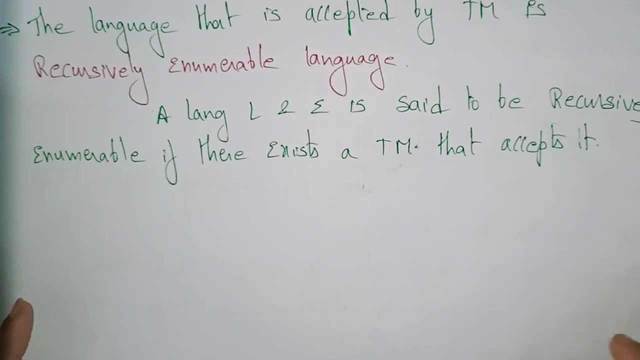 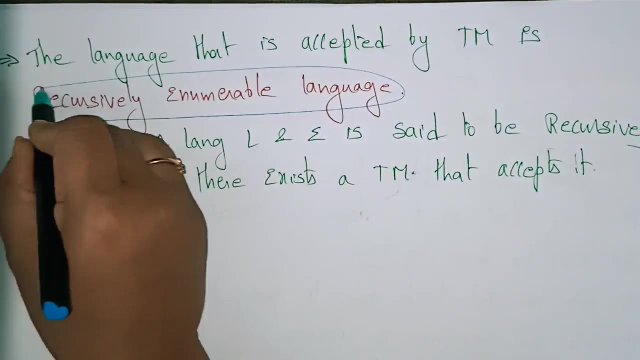 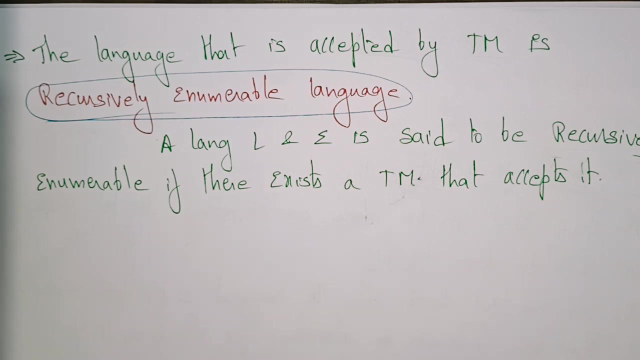 okay, and this is also one argument. and another argument here is: the language that is accepted by a turing machine is recursively enumerable language. that we already said in the definition. whatever the language that is accepted by the turing machine is recursively enumerable language. here the language and Sigma is 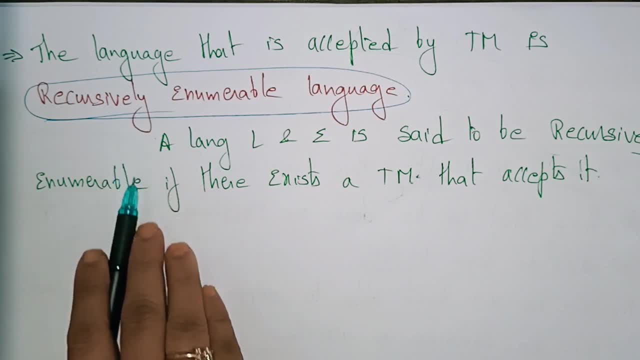 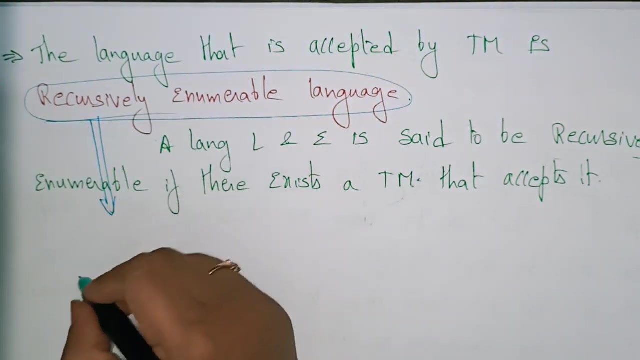 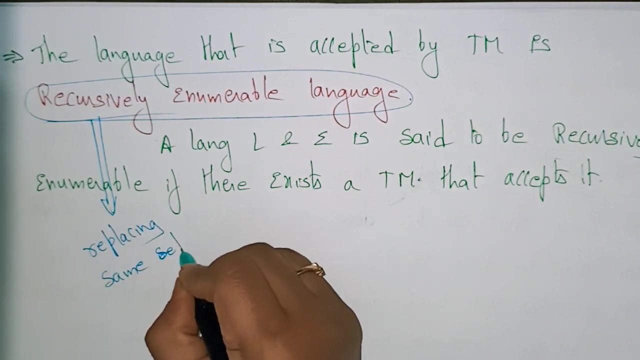 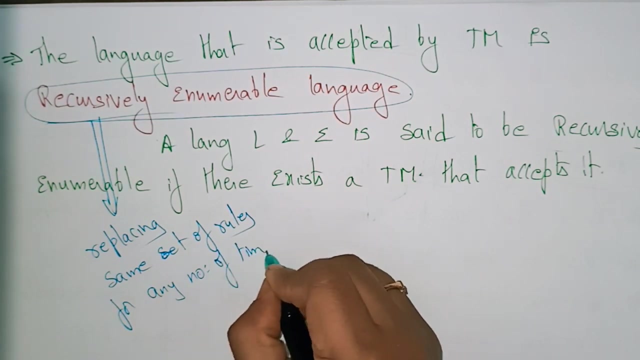 said to be recursively, okay. it is said to be recursively enumerable if there exists a turing machine and that accepts it, okay, okay. so when you can say that the language is recursively, okay. recursive means here: a recursive means nothing but replacing. replacing same set of rules, same set of rules for any number of times we are. recursively means we are. 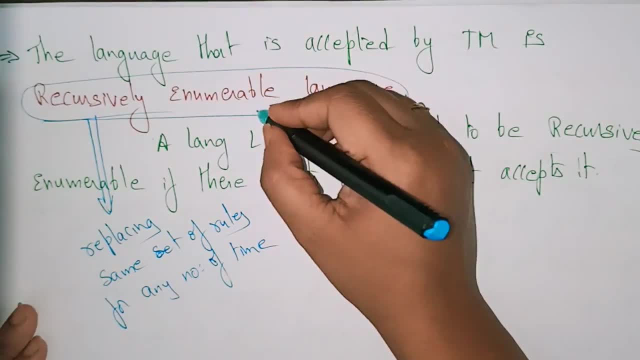 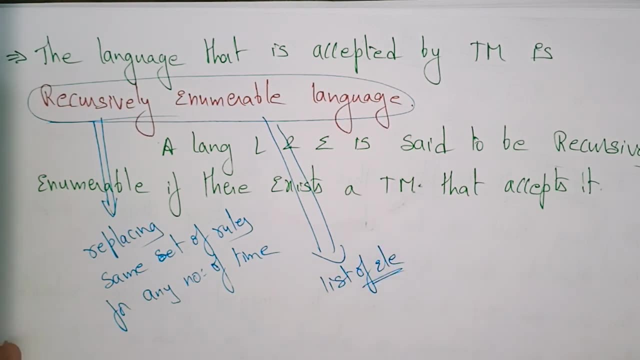 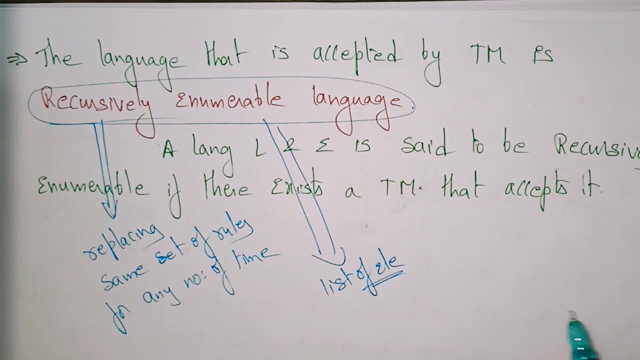 just replacing the same set of rules any number of times. then what about the enumerable enumerable rules? enumerable means nothing but the list of elements. list of list of elements. okay, so the language that is accepted by the turing machine is recursively enumerable language, so a that is what is the recursive enumerable, and it's nothing. 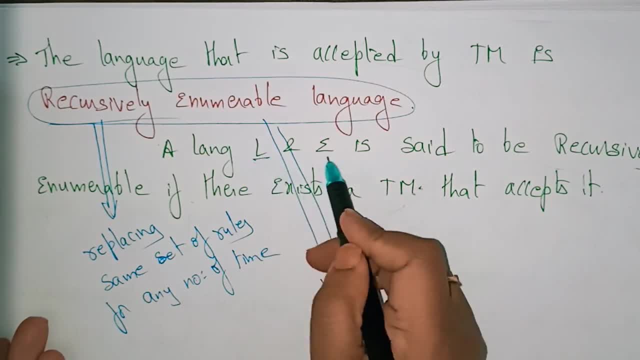 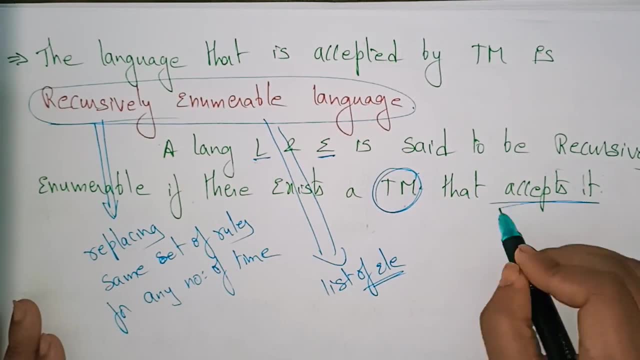 but it is a language, a language L, and Sigma, that is an input symbol, is said to be recursively enumerable. if there exists a turing machine, that turing machine has to be accepted. okay, so this is a recursive enumerable language, and so this is the turing machine thesis. thank you,